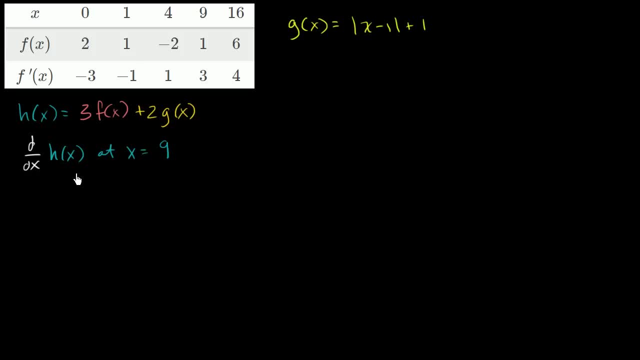 with the notation of writing this: the derivative of h of x with respect to x at x equals nine. this is equivalent. this is equivalent to h. let me do it in that blue color. it is equivalent to h prime and the prime signifies that we're taking the derivative. 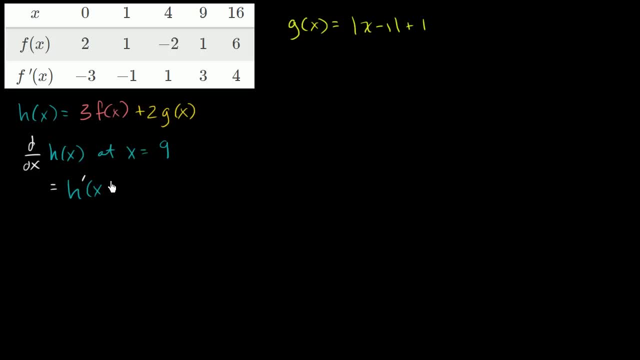 h prime of h prime of x when x equals nine. so h prime of nine is what this really is. Actually, let me do this in a different color. So this is h prime of nine. So let's think about what that is. 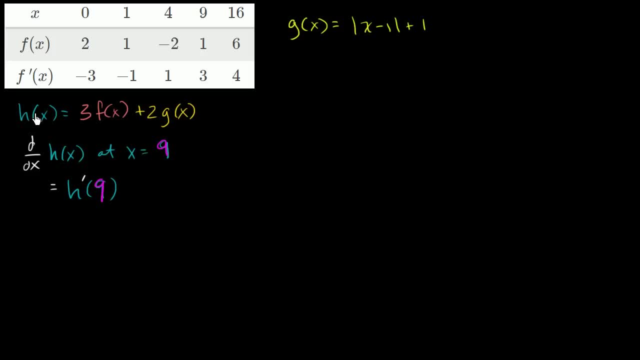 Let's take the derivative of both sides of this expression to figure out what the derivative with respect to x of h is. So we get derivative. let me do that same white color Derivative with respect to x, with respect to x of h of x. 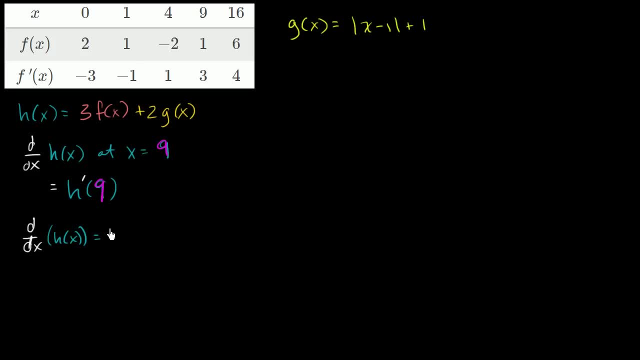 h of x is going to be equal to the derivative with respect to x of all of this business. So I could actually just well- I'll just rewrite it- Three times f of x plus two times g of x, plus two times g of x. 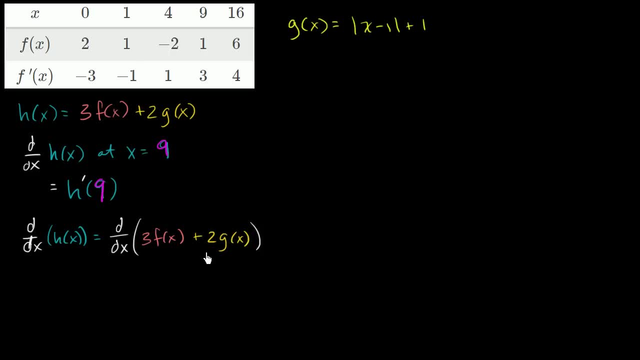 Now this right over here: the derivative of the sum of two terms. that's going to be the same thing as the sum of the derivatives of each of the terms. So this is going to be the same thing as the derivative with respect to x. 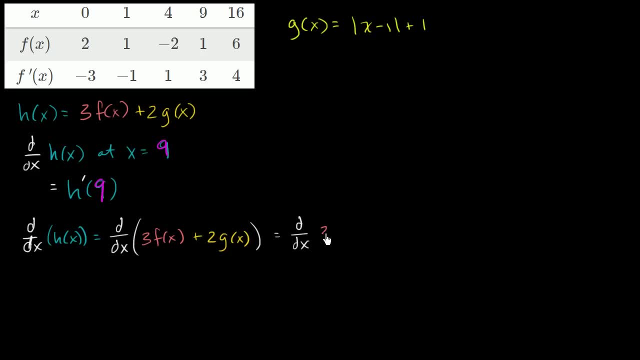 of three times- let me write that a little bit neater- three times f of x, plus the derivative, with respect to x, of two times g of x. two times g of x, Now the derivative of a number, or I guess you could say a scaling factor, times a function. 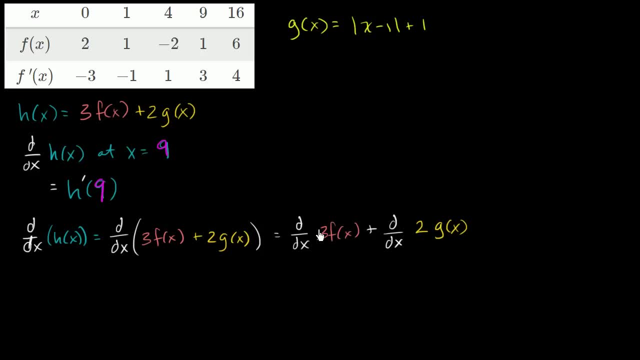 the derivative of a scalar times a function is the same thing as the scalar times, the derivative of the function. What does that mean? Well, that just means that this first term right over here, that's going to be equivalent to three times the derivative. 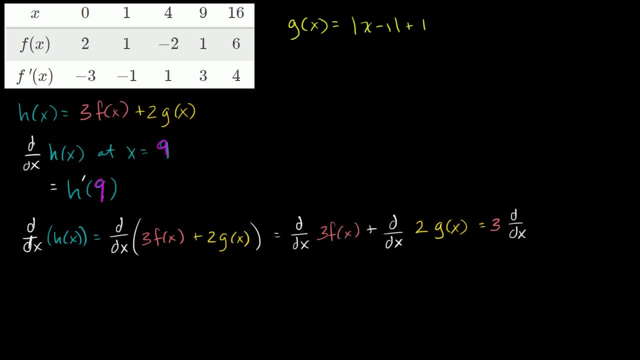 with respect to x of f of our f of x, plus this part over here, is the same thing as two- let me make sure I don't run out of space here- plus two times the derivative with respect to x. the derivative with respect to x of g of x. 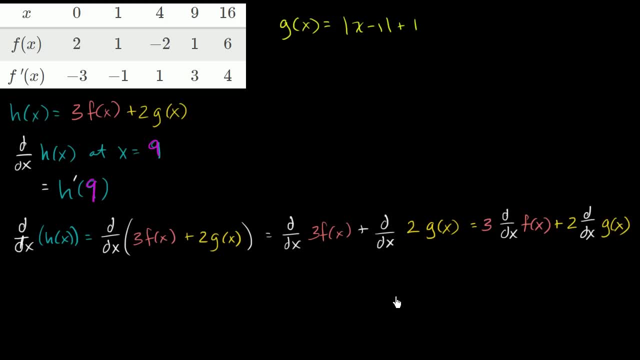 of g of x, of g of x. So the derivative of h with respect to x is equal to three times the derivative of f with respect to x, plus two times the derivative of g with respect to x. And if we wanted to write it, 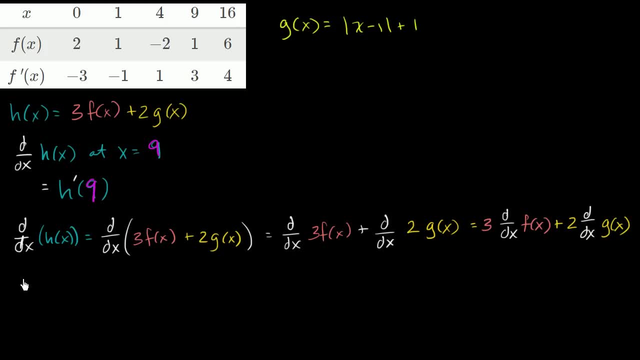 in this kind of prime notation. here we could rewrite it as: h prime of x is equal to three times f prime of x. so this whole, this part right over here, that is the same thing as f prime of x. So it's three times f prime of x. 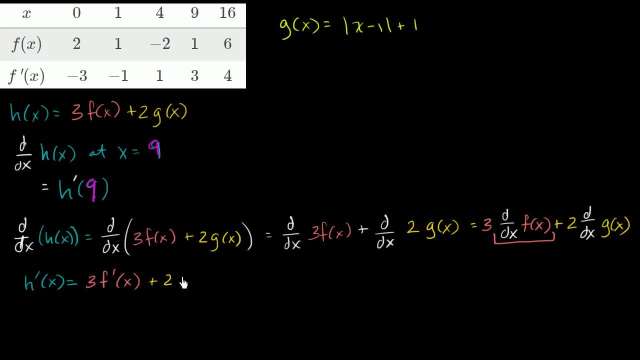 plus two times g prime of x, plus two times g prime of x, And once you kind of And once you kind of And once you kind of are more fluent with this property, the derivative of the sum of two things. 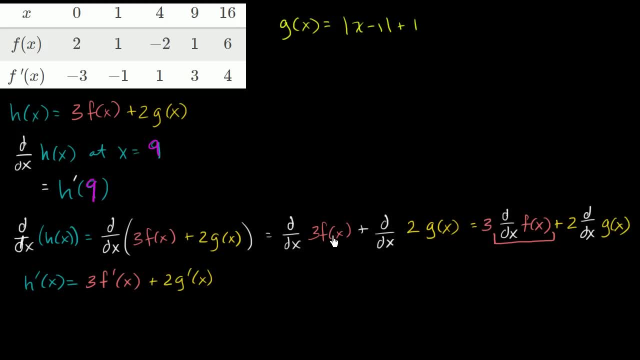 is the sum of the derivatives and the derivative of a scalar times something is the same thing as the scalar times, the derivative of that something. you really could have gone straight from straight from here to here pretty quickly. Now, why is this interesting? 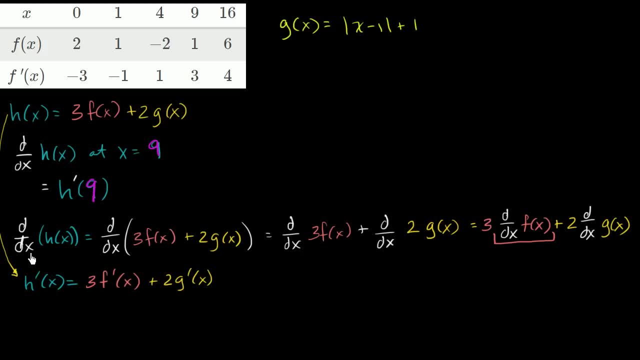 Well, now we can evaluate this function when x is equal to nine. So h prime of nine is the same thing as three times f prime of nine plus two times g prime of x, plus two times g prime of nine. Now what is f prime of nine? 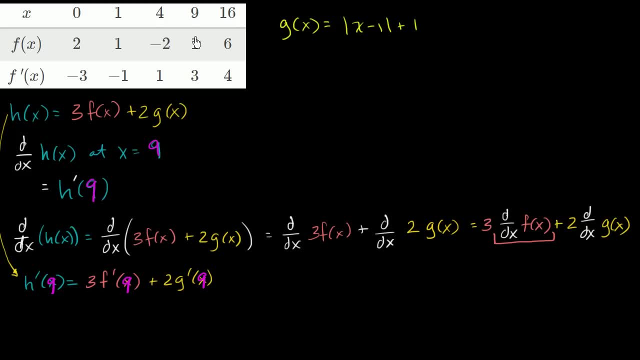 The derivative of our function f when x is equal to nine. Well, they tell us, when x is equal to nine, f of nine is one, but more importantly, f prime of nine is three. So this part right over here evaluates that part's three. 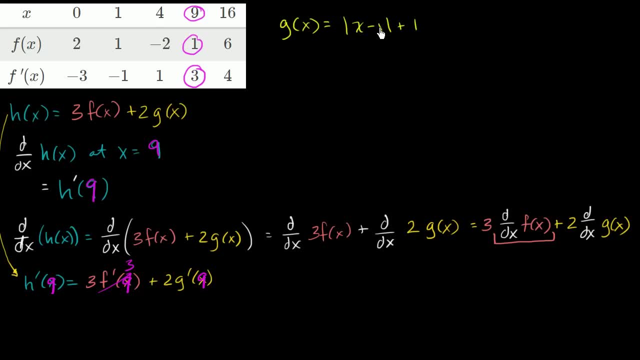 But what's g prime of nine? So let's look at this function a little bit, a little bit more closely. So there's a couple of ways we could think about it. Let's actually let's try to graph it Now. I think that could be interesting. 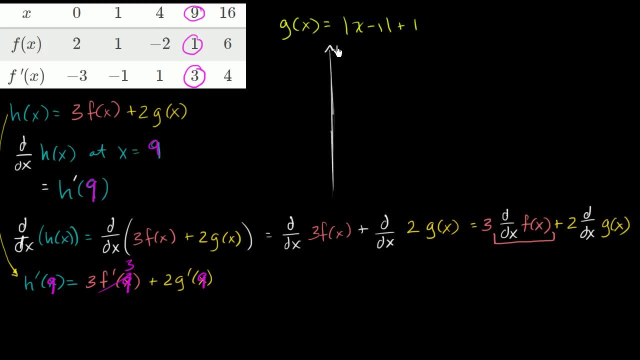 Just to visualize what's going on here. So let's say that's our y-axis and this right over here is our x-axis. Now, when does an absolute value function like this? when is this going to hit a minimum point? Well, the absolute value of something. 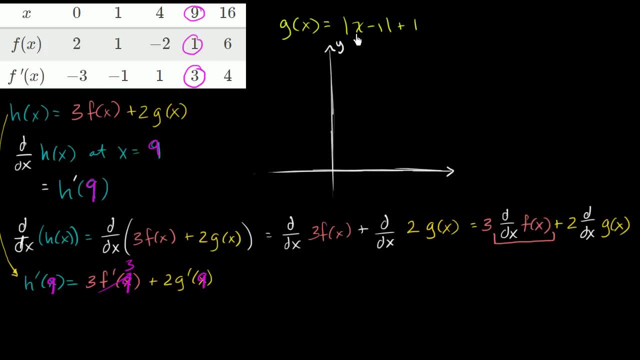 is always going to be non-negative. So it hits a minimum point when this thing, when this thing is equal to zero. Well, when is this thing equal to zero? When x equals one, this thing is equal to zero. So we hit a minimum point when x is equal to one. 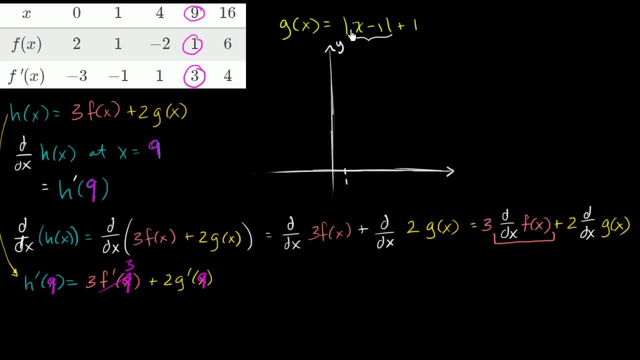 And when x equals one, this term is zero. absolute value of zero is zero, G of one is one. So we have this point right over there. Now, what happens after that? What happens for x greater? What happens for x greater than one? 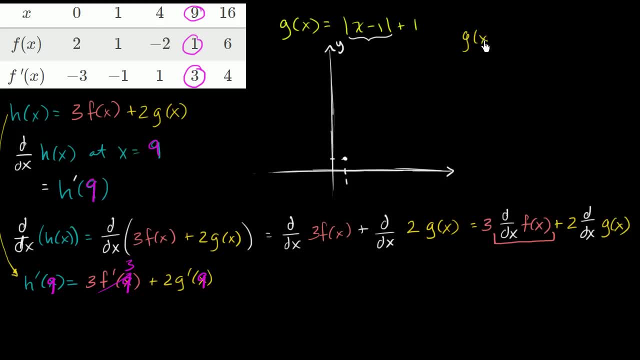 Actually, let me write this down. So g of x is equal to and. in general, whenever you have an absolute value or a relatively simple absolute value function like this, you could think of it, you could break it up into two functions, or you could think about this function. 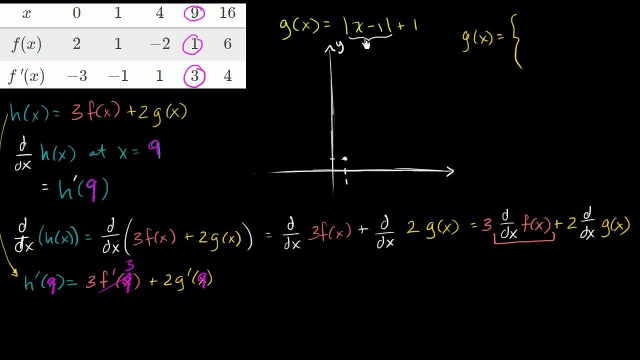 over different intervals: when the absolute value is non-negative and when the absolute value is negative. So when the absolute value is non-negative, that's, when x is greater than or equal to zero, x is greater than or equal to zero And when the absolute value is non-negative. 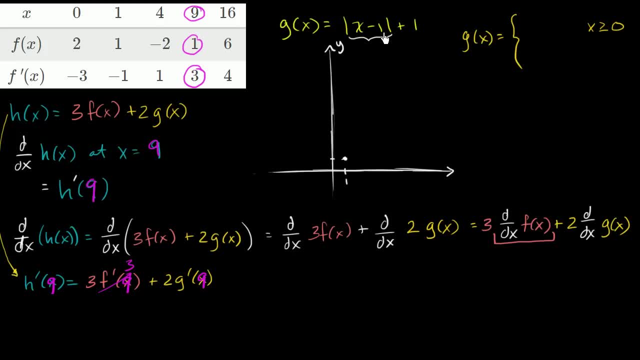 if you're taking the absolute value of a non-negative number, then it's just going to be itself: The absolute value of zero is zero. Absolute value of one is one. Absolute value of 100 is 100. So then you could ignore the absolute value. 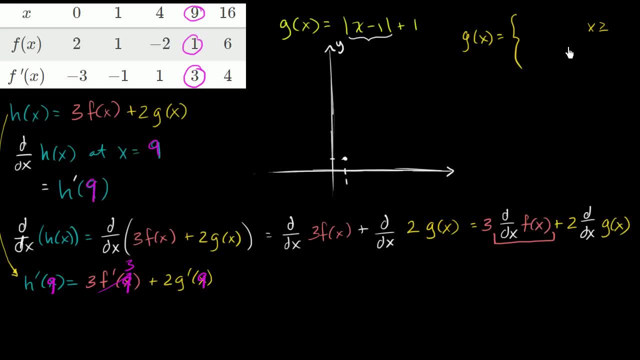 for x is greater than or equal to, oh, not greater than or equal to zero. for x is greater than or equal to. x is greater than or equal to one. x is greater than or equal to one. this thing right over here is non-negative. 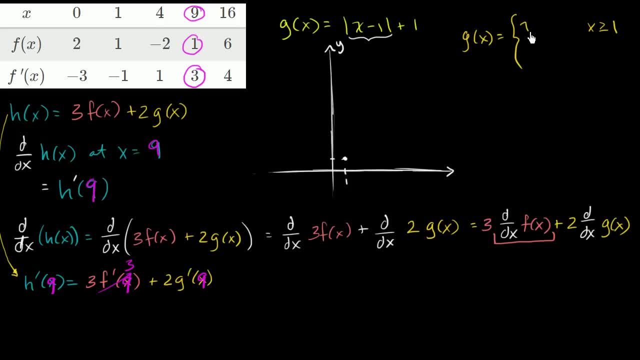 And so it'll just evaluate to x minus one. So this is going to be x minus one plus one, which is the same thing as just x Minus one plus one. they just cancel out Now when x when this term. 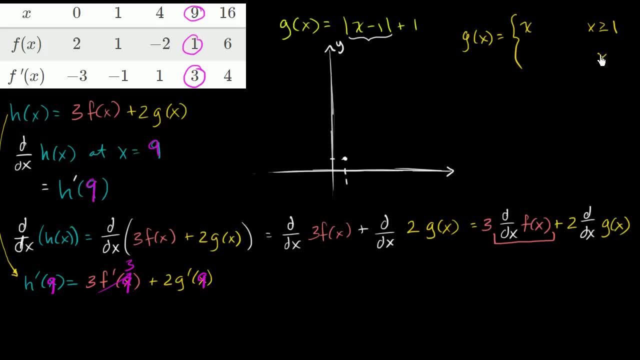 right over here is negative, and that's going to happen for x is. this is going to happen for x is less than one. well then, the absolute value is going to be the opposite of it. You give me the absolute value of a negative number. 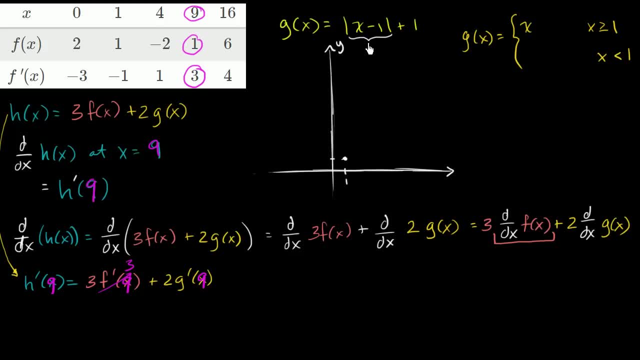 it's going to be the opposite. Absolute value of negative eight is positive eight, So it's going to be the negative of x minus one is one minus x plus one, Or we could say two minus x, Two minus x. Now. so for x is greater than or equal to one. 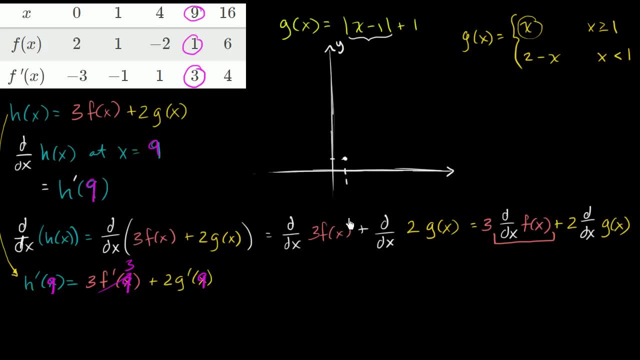 we would look at this expression: Now, what's the slope of that? Well, the slope of that is one. So we're going to have a curve that looks like, or a line. I guess we could say that looks like this. 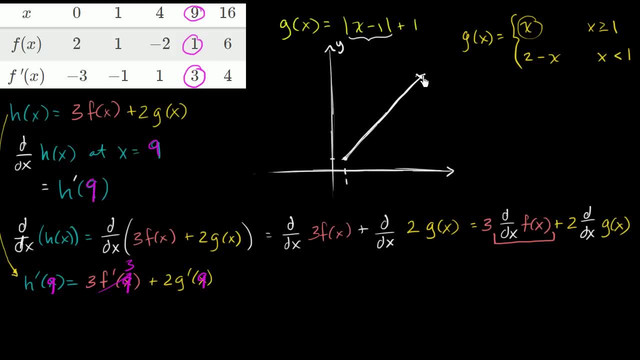 That looks like this For all x's greater than or equal to one. So the important thing, remember, we're going to think about, we're going to think about the slope of the tangent line when we think about the derivative of g. So slope is equal to one. 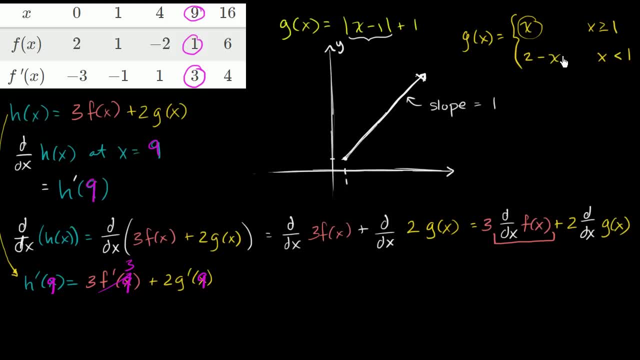 And for x less than one. well, our slope- now, if we look right over here, our slope is negative. Our slope is negative one. So it's going to look like this, It's going to look like that, But for the point in question. 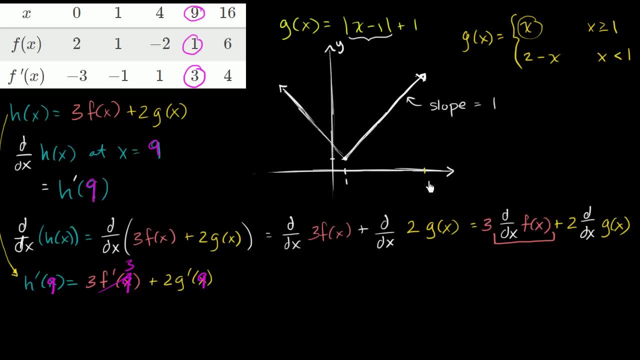 if we're thinking about g prime of nine. so nine is someplace out here. So what is g prime of nine? So g prime of nine. let me make it clear this graph right over here, this is the graph of g of x. 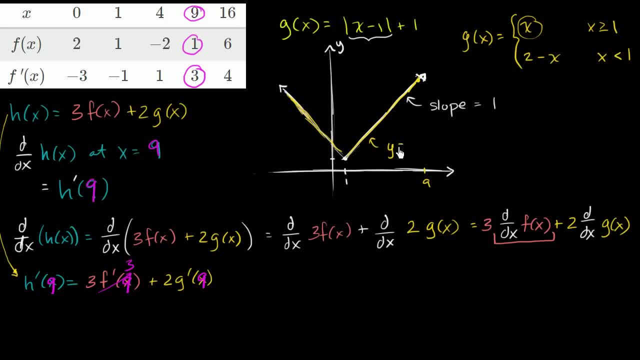 Or we could say y. this is the graph. y equals g of x, Y is equal to g of x. So what is g? prime of nine? Well, that's the slope. when x is equal to nine, Well, the slope is going to be equal to one. 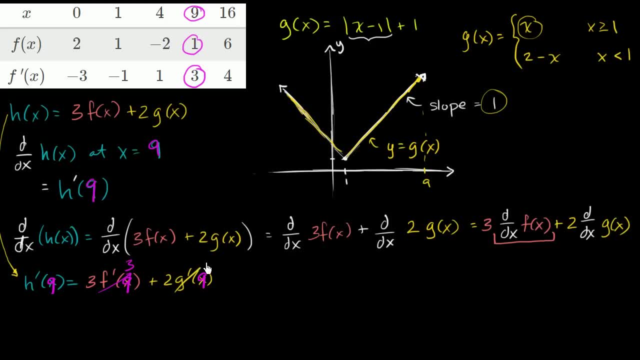 So g prime of nine, g prime of nine is one. So what does this evaluate to? This is going to be three times three. So this part right over here is nine Plus two times one Plus two, which is equal to 11.. 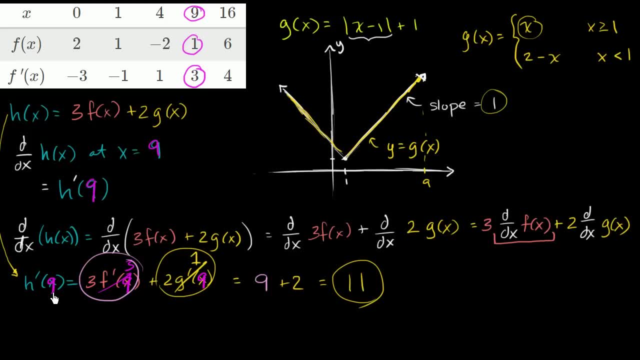 So the slope of the tangent line of h, when x is equal to nine, is 11..